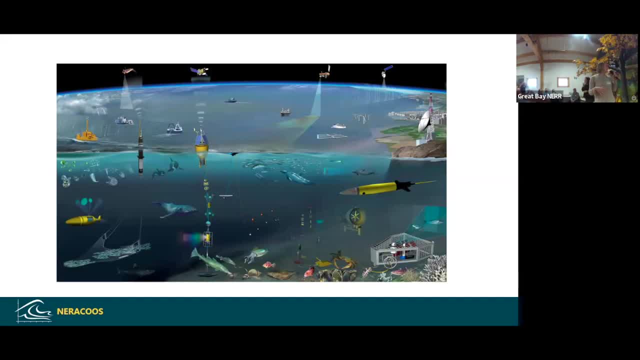 So what I'm here speaking about today is kind of our evolving marine life program. So I put this figure up here just because it's kind of an interesting image And it shows all of the different, diverse ways we can monitor the ocean and coastal environment- everything from remote sensing to buoys and then down. 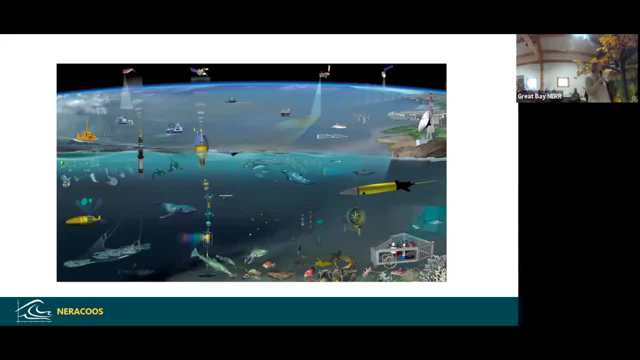 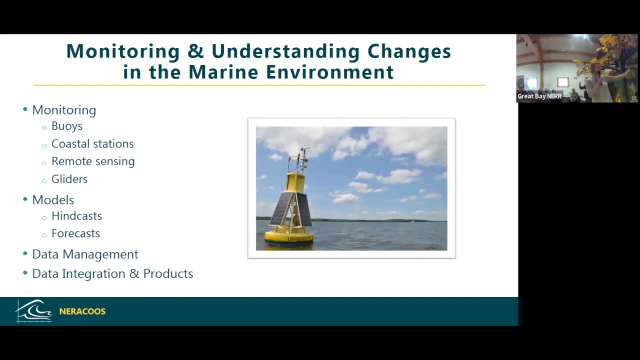 Throughout the water column and how this interacts with our marine life and how we monitor this marine life system. So in the Northeast, this is a picture of the Great Bay buoy, which some of you might know, which Tom Gregory operates, and the team at UNH. So this is an asset that we help to support. 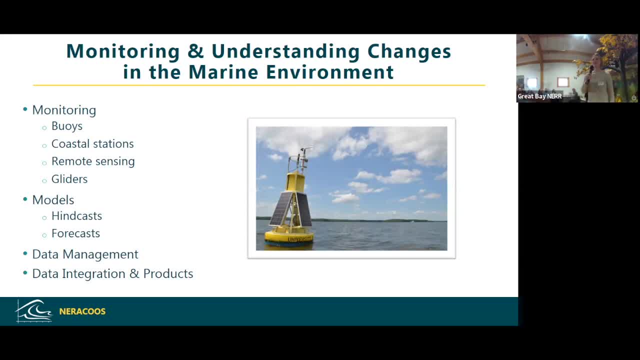 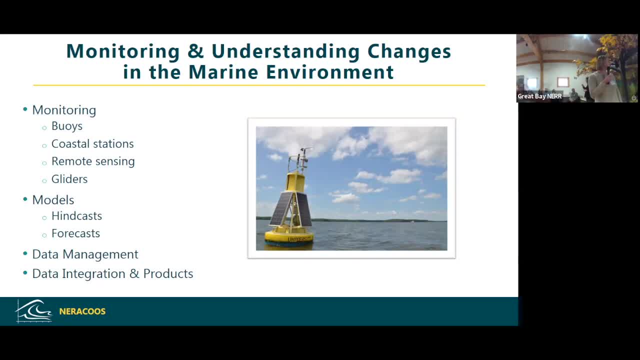 in addition to buoys, we support a number of coastal stations. some work with remote sensing gliders. We have a number of buoys offshore throughout the Gulf of Maine. Also connected to the system are modeling systems, the Northeast Coastal Ocean Forecast Systems and all of this. 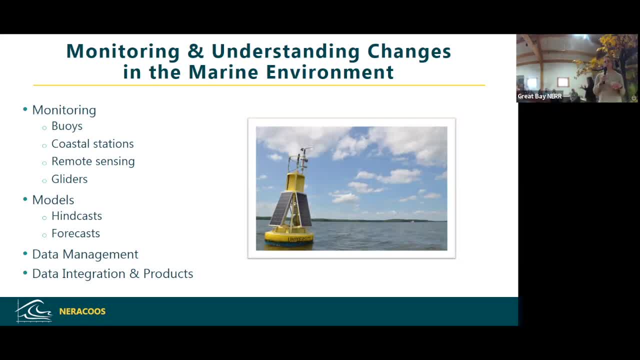 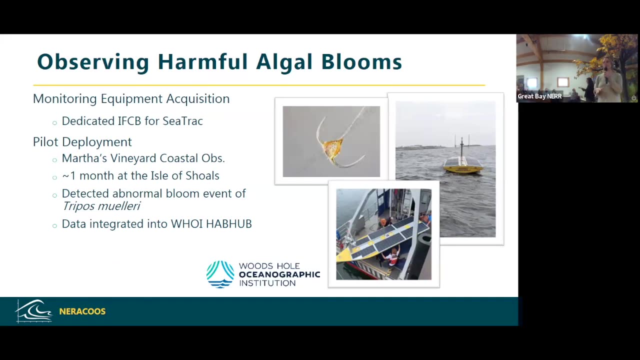 information comes together through consistent data management standards that makes it accessible to all of you, and through various different products or integration. So, thinking about how we monitor the marine system, we use that core observing system as the backbone and we have chosen to evolve it in certain ways, based on core sentinel indicators of change or key locations. One of the 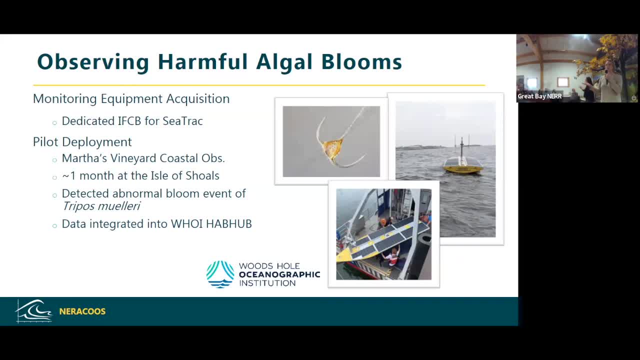 key priorities- and this is an evolving program with NCOSS and IUSE- is implementing a sustained ocean observing system to monitor harmful algal blooms. Right now we have a lot of research efforts. there's a lot of great work that Liz and others are doing here in Great. 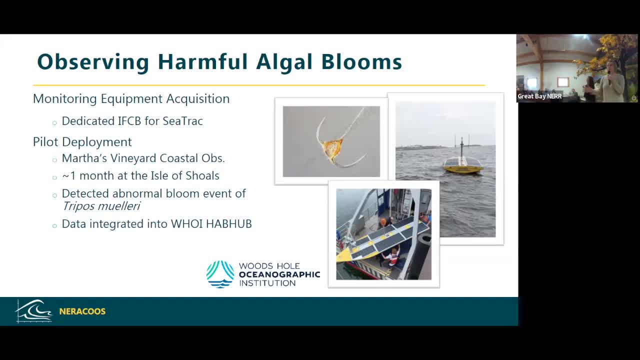 Bay More broadly. how do we understand harmful algal blooms throughout the region? We are working with Woods Hole Oceanographic Institution. You can see this autonomous vessel here being loaded onto the Gulf Challenger and underneath this is an imaging flow site About that can take pictures of the critters through this water column and there's a picture. 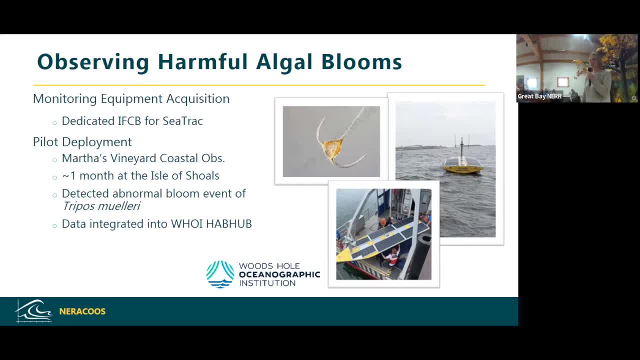 of the, the tripos blue from the summer. Cameron will be speaking about that more later today, but this is a pilot program to test this new technology to get into some of these more remote locations. This summer it was deployed for a month out at the Isle of Shoals. We are hoping that this 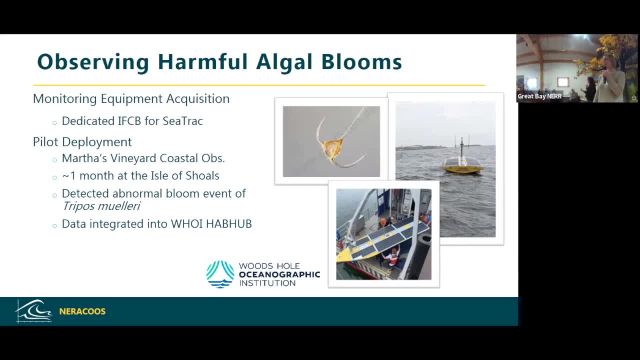 can be part of a rapid response to harmful algal blooms in locations that are difficult to access, and it's a new technology that we're working on. And then we're working on the water quality of the water that we're testing to deploy in new locations. We're also looking at key sentinel. 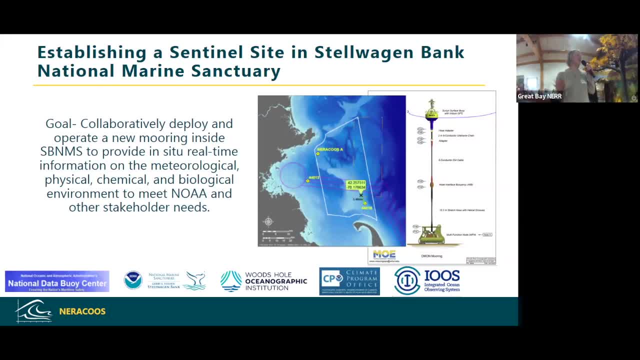 locations And I realize I've moved a little bit beyond New Hampshire, but there are applications potentially throughout the region of how we monitor the water column. So Stellbegen bank has a National Marine Sanctuary, has a number of management priorities In addition to it's a really 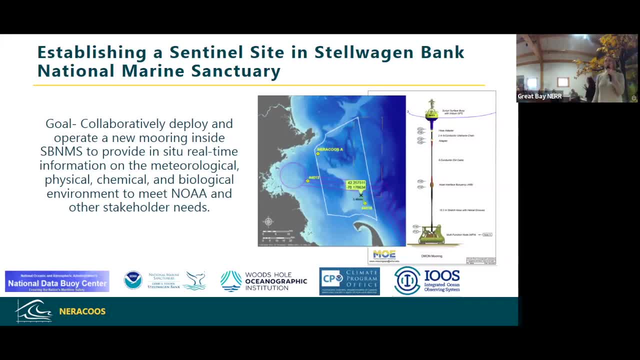 popular place for tourism, for fishing. There's a lot of convergence of multiple needs here and so we're working on that. we are kicking off a new effort, in partnership with all the folks identified here on the bottom, to co-locate and build a new buoy that will meet all the needs of the sea. state information. 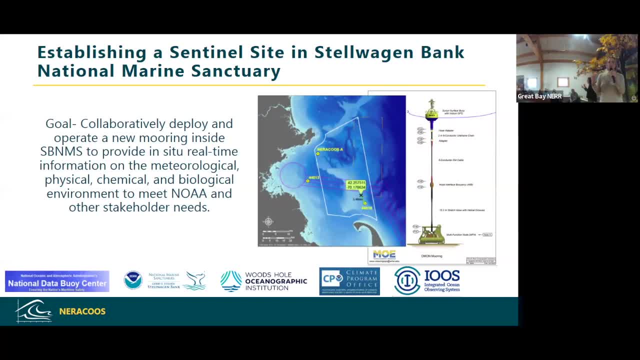 the information that the weather service needs, as well as that's needed by the sanctuary. So something that's really unique about this is that we will be integrating real-time passive acoustic information into this buoy design, which is really unique and something really new, and 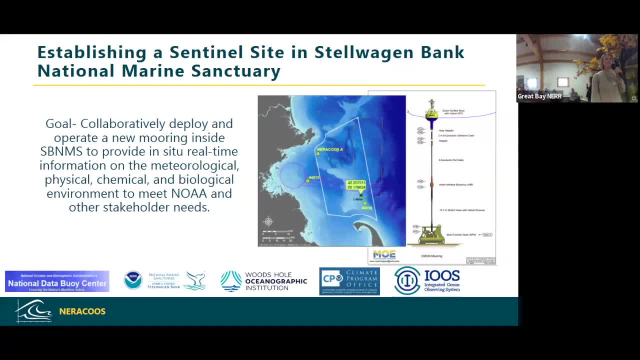 novel, since these chains and these buoys are out there all the time. They make a lot of noise. So what we're hoping to do is to integrate passive acoustic monitoring as well as a number of other sensors, so we can really start to look at the system more holistically to understand. 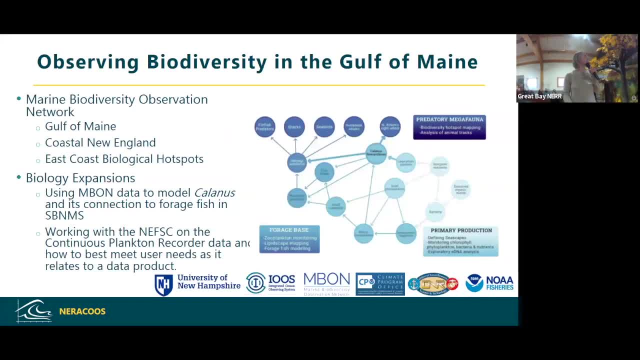 the changes that are occurring. Also, we are working with a number of folks- and Nathan's in the room too. We're looking at marine biodiversity, doing this in a number of different ways. We are working with a few different projects. As you can see, collaboration is the name of the game for. 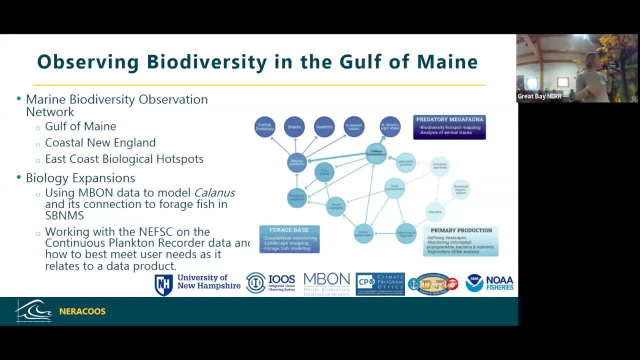 every thing we do. So one of those is through monitoring Calaniths and Marchicus throughout the Gulf of Maine and what that means to the food web, As I said, working with Nathan and the Colts of New England MBOM program and then also looking at tag species and identification. 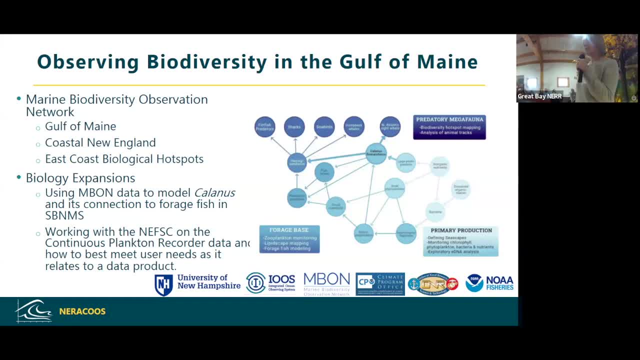 of biological hotspots And we have some new evolutionists. We've been working with the Calaniths and Marchicus project in the coming years And one of these is to take some of this plankton data that we've been collecting through this MBOM work, and Cameron is leading up this. 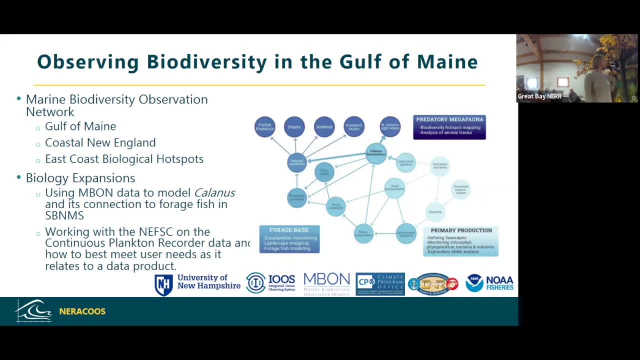 modeling effort to better understand how Calaniths moves throughout the food web in the Gulf of Maine and the implications to the forage fish at Stillwang and Bank. So really thinking about all of these various components to the ecosystem and the different levels and how we can really think, 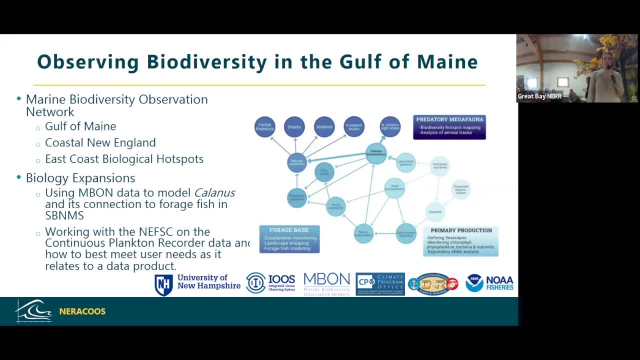 about the system more holistically. Additionally, we're working with the Northeast Fisheries Science Center on plankton and trying to think about what kind of data products do we need to really understand the changes that we're seeing in plankton throughout the region? So we will be 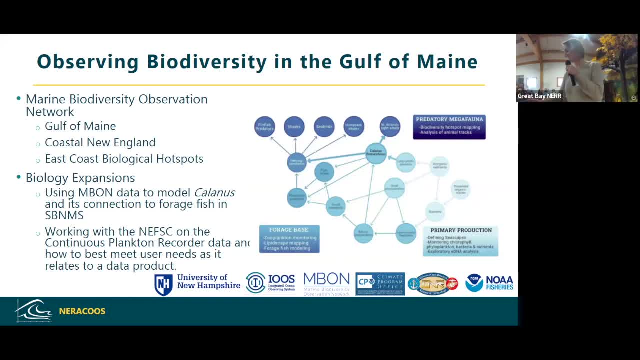 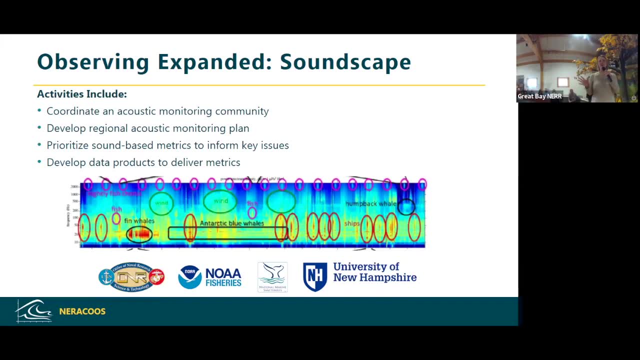 hosting a workshop this spring. If you're interested, please let me know. Okay, I'm getting close on time And this is my last slide. Also really exciting is the expansion of thinking about soundscape information, For in the Northeast, luckily, there's been a really wonderful baseline soundscape information collected And there's going.